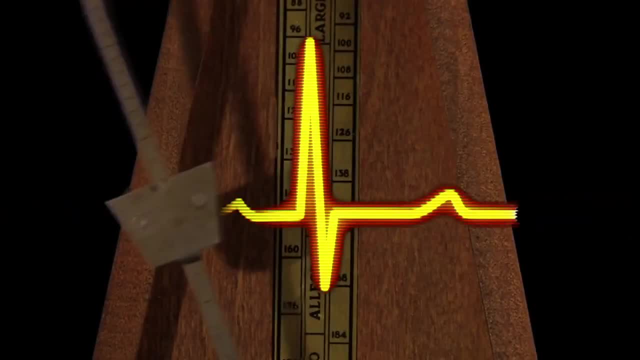 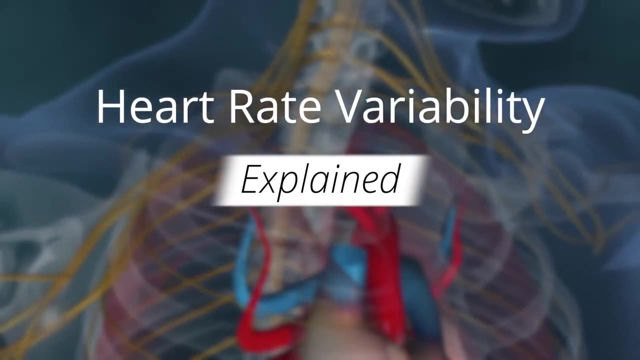 If you think your heart beats at a regular interval like a metronome, think again. We have a natural variability in the spacing between our heartbeats and this phenomenon is called heart rate variability, and HRV for short. It says a lot. 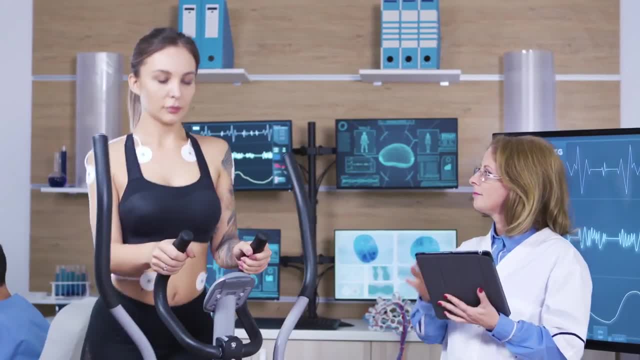 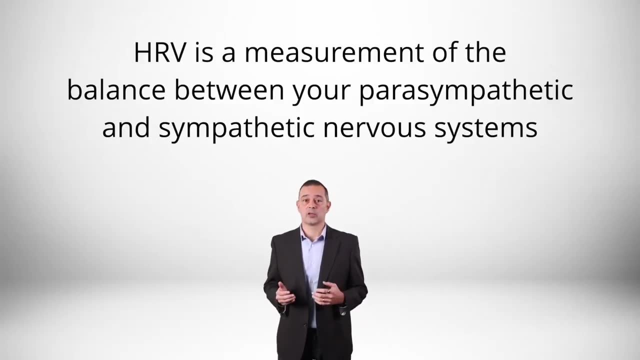 about our body systems, which is why athletes and health enthusiasts alike have been so interested in this and why you should be too. Simply put, HRV is a measurement of the balance between your parasympathetic and sympathetic nervous systems. These two systems make up the autonomic nervous. 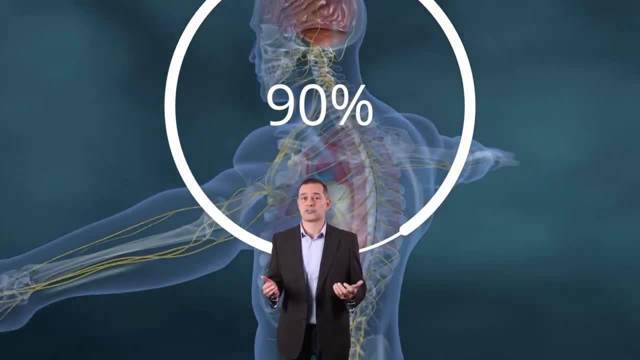 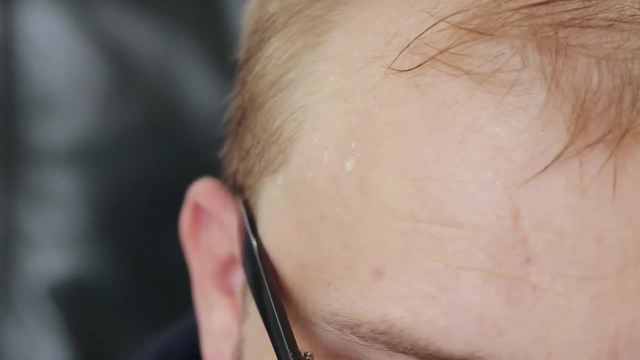 system which handles about 90% of the body's involuntary functions. The sympathetic nervous system is what kicks into gear when we're stressed or in danger. We sweat, our heart rate goes up and the interval between our heartbeats goes down. Our body is either primed to fight or flight. 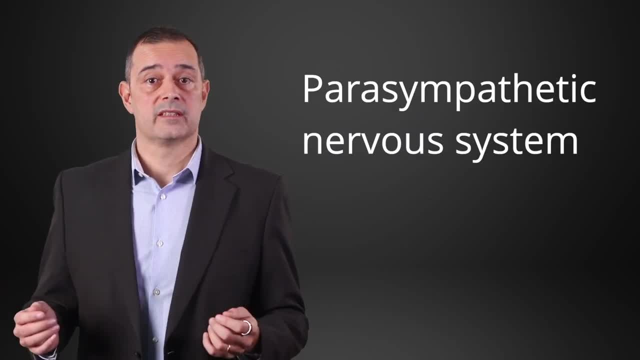 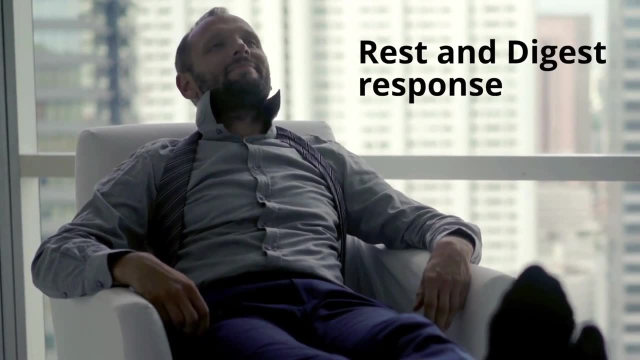 The parasympathetic nervous system is pretty much the opposite and it functions like a brake by disabling the sympathetic nervous system Called the rest and digest response. it activates when we're in a relaxed state and engages processes such as the production of saliva and peristalsis. 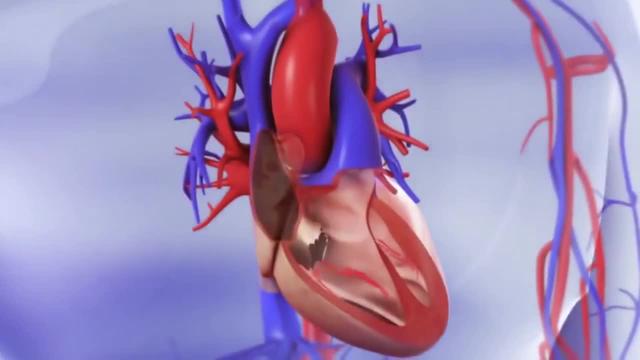 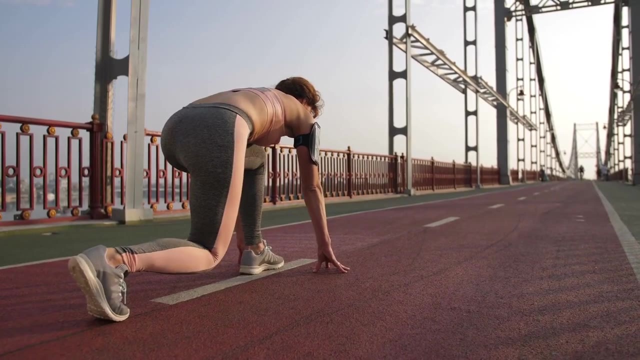 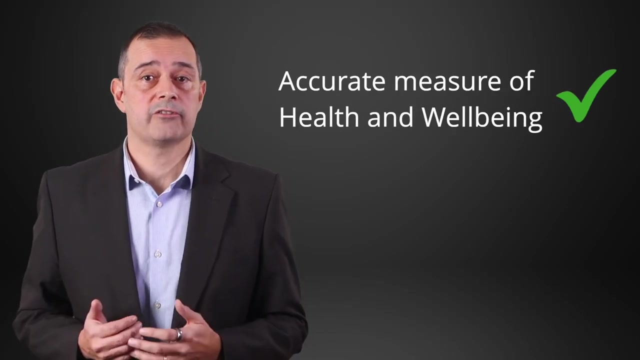 It slows the heart rate with greater intervals between beats. When, in balance, your heart produces a high HRV through a more variable heart rate. The more variable your heart rate, the more you can readily respond to your environment and switch gears between these two systems. It's one of the most accurate measurements. 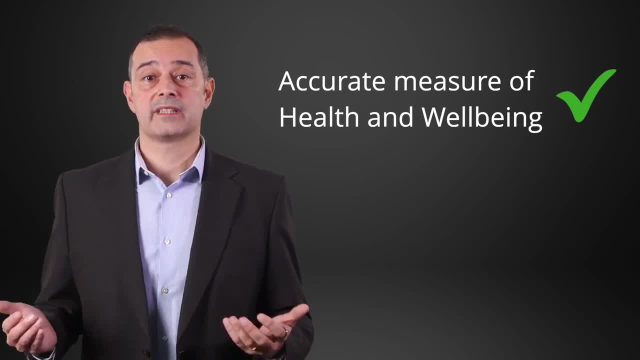 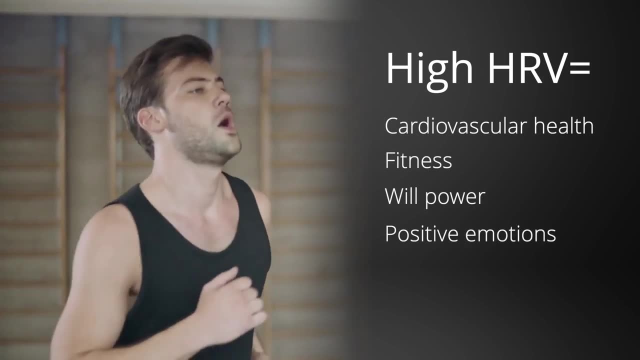 of overall health that we can get without taking blood tests or body scans. High HRV is an indication of cardiovascular health, fitness, willpower and positive emotions and your capacity to handle stress. The lower your HRV, the less capacity for stress that you have in your body. 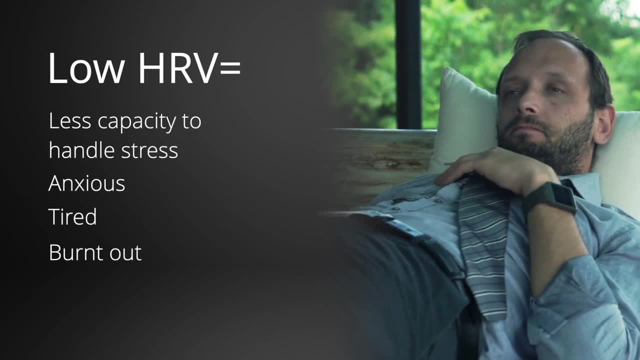 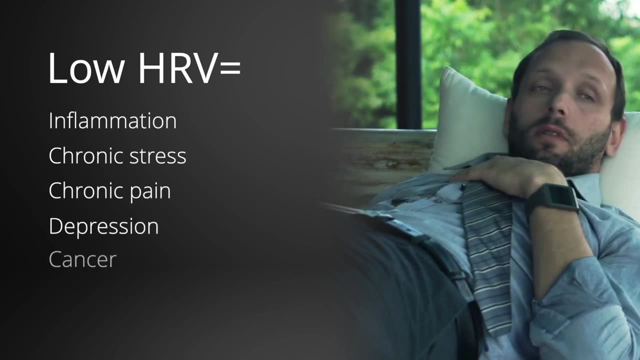 so, the more likely you are to feel anxious, tired or burnt out at the end of the day. Low HRV is also related to inflammation, chronic stress, chronic pain, depression, cancer and low emotional flexibility. HRV is used in professional sports. 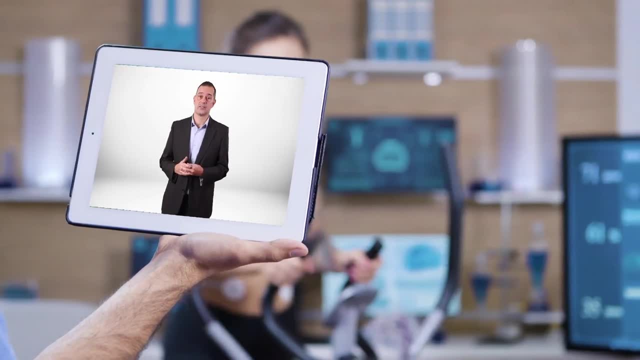 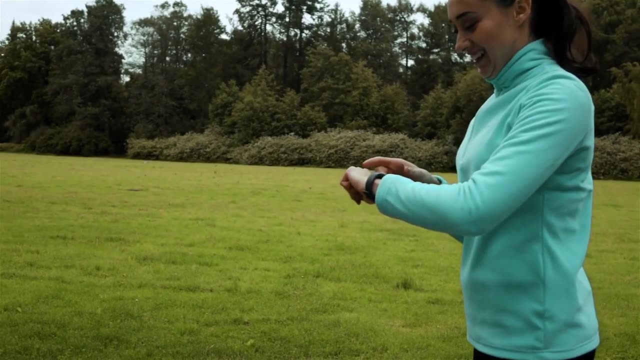 sports to predict injury and by forward-thinking doctors to diagnose disease. Many smartwatches now can indicate your stress levels by measuring HRV through your wrist pulse. It's a huge predictor of persistence and self-control and it increases when exerting self-regulation. This mechanism is called the pause and plan response. By changing our physiology, we can manipulate our HRV, and there are several ways to improve your heart rate variability. The simplest way to improve your HRV is through breathing at a rate which is called cohesion. 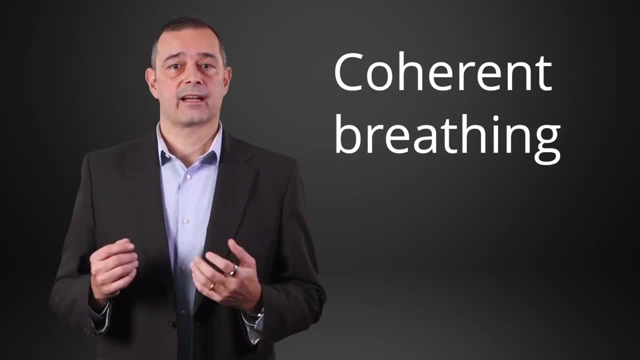 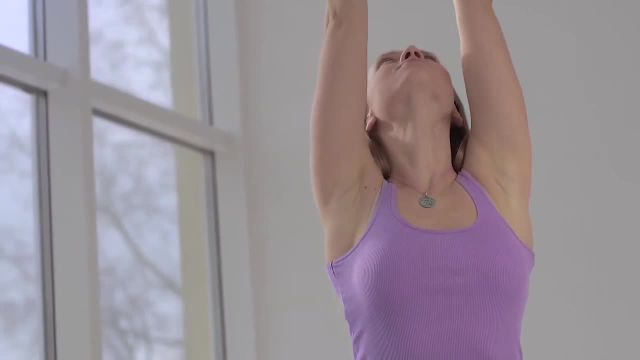 Coherent breathing. By slowing down your breathing, you can activate the parasympathetic nervous system and raise your HRV, which causes your heart rate and blood pressure to synchronize with your breathing, resulting in a state that the HeartMath Institute calls coherence. 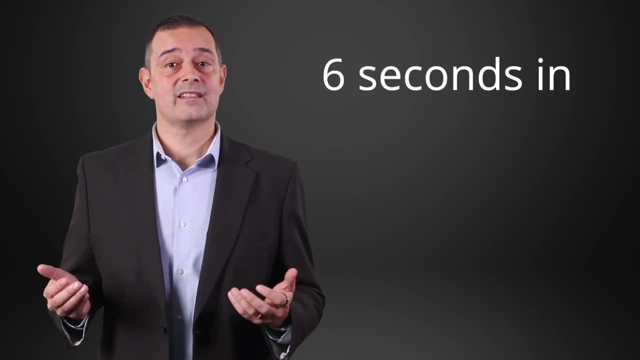 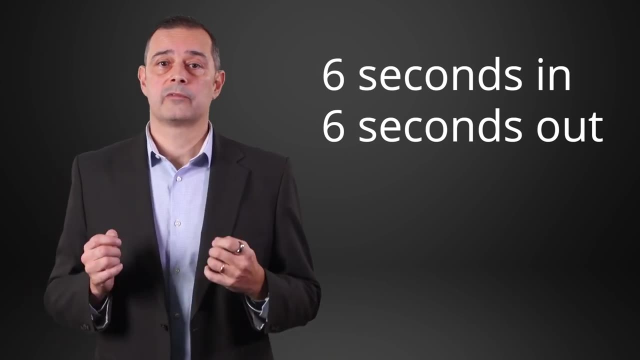 For most people, the optimal breathing rate will be around six seconds in, six seconds out. Five breaths a minute might feel slow, particularly if you do suffer with stress or anxiety, but you will feel the benefits immediately Doing a minimum of 10 minutes of this breathing every day. 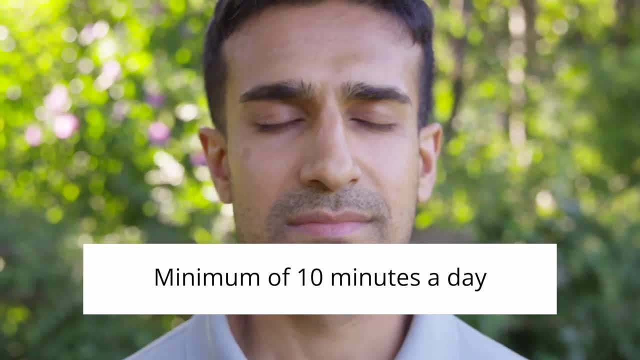 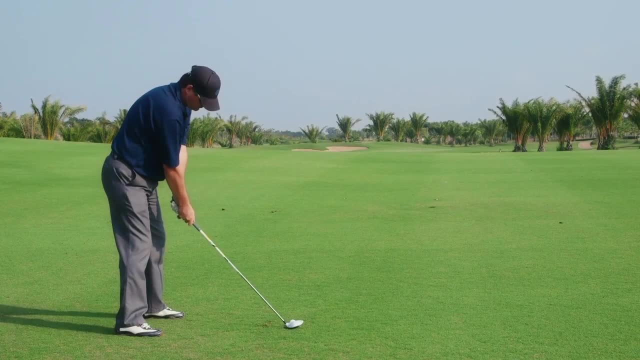 you can develop the skill of producing the state of coherence at any time. Activating this state, you can get into the zone, so to speak, and increase your performance for single actions such as swinging a golf club or presenting to a group. 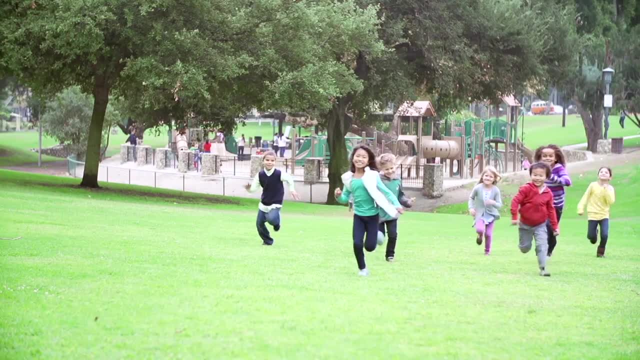 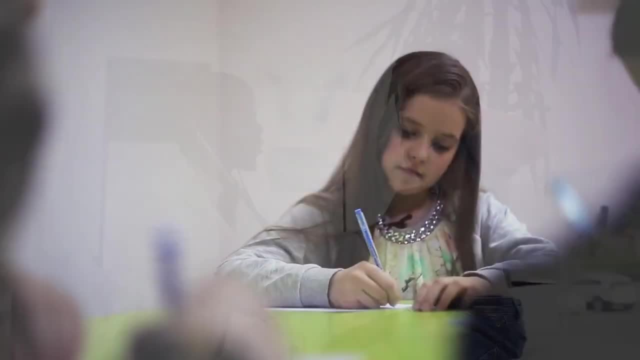 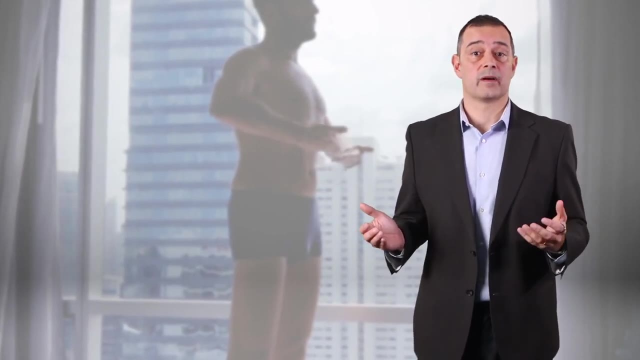 HRV training is shown to be incredibly beneficial for children with overactive sympathetic nervous systems and things like belly aches. After a few weeks of daily training they show massive improvements in their baseline HRV and can function much better. Some autoimmune conditions related to the gut have been helped by this type of training. 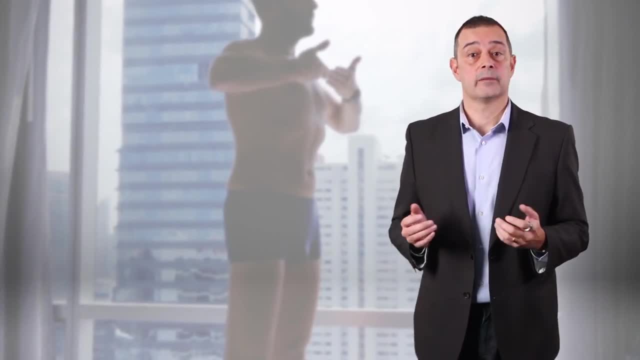 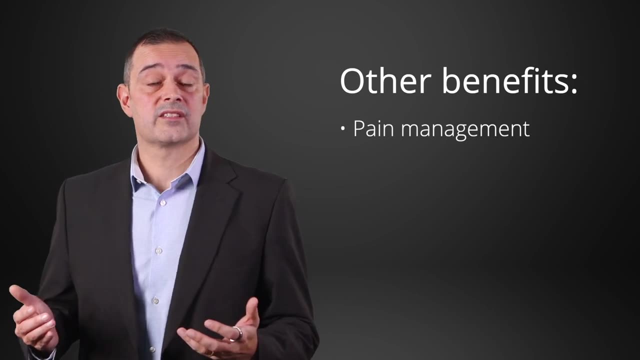 as well as our gut. permeability is closely related to the parasympathetic nervous system. Other benefits of HRV breathing include improved pain management in conditions such as fibromyalgia and chronic muscle pain. It can also help with asthma, depression, hypertension. 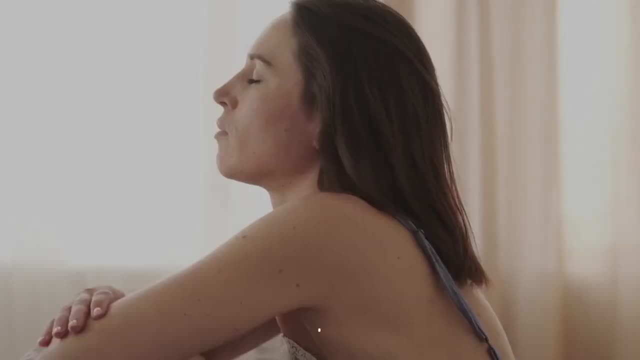 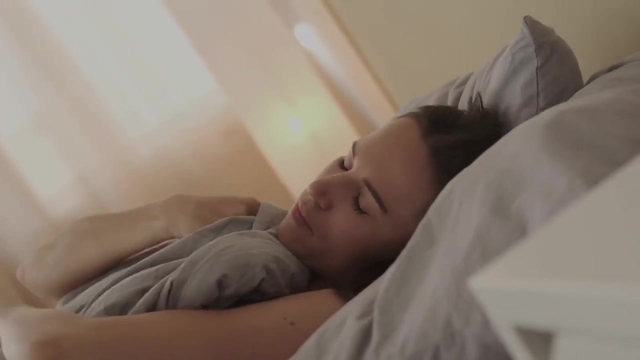 and self-control, and so is great for stress management. What are the benefits of HRV? breathing Around 20% of people- most people- feel sleepy from following this breathing rhythm, which makes it a great tool for getting high quality sleep every night. 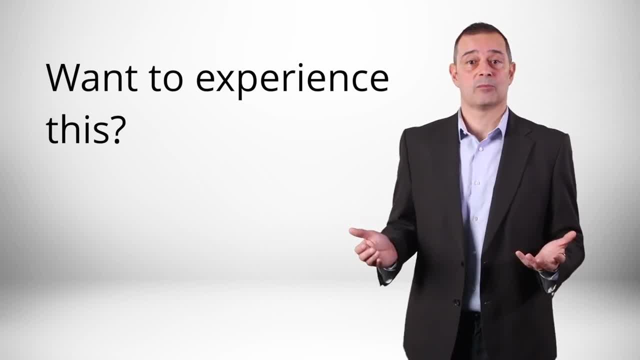 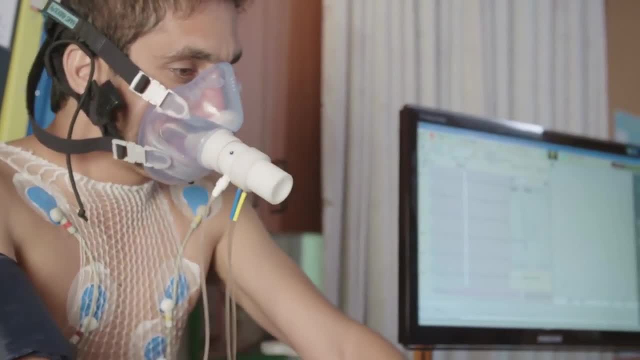 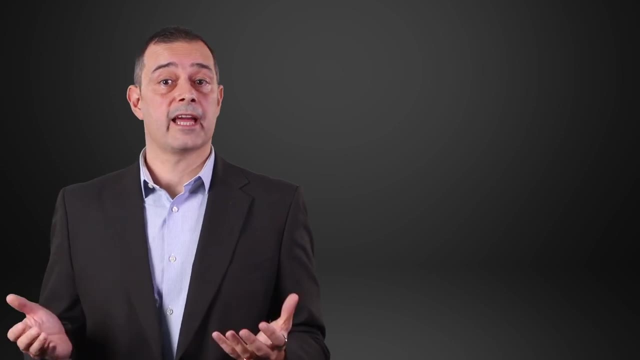 If you want to experience this state of coherence, you'll find a video here on my channel. The interest in HRV has increased substantially in the past decade and several consumer technologies have emerged to help measure your personal HRV metrics. The most accessible way to accurately measure your HRV is to use a free app called Welltory. 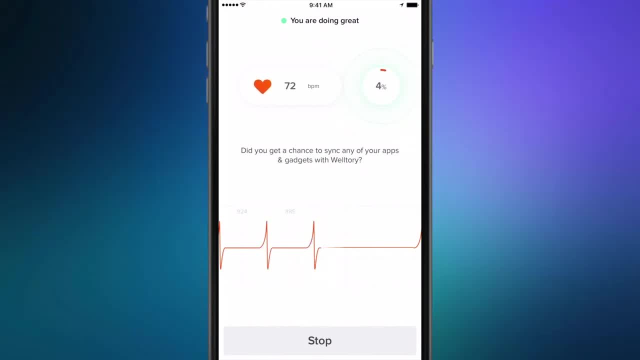 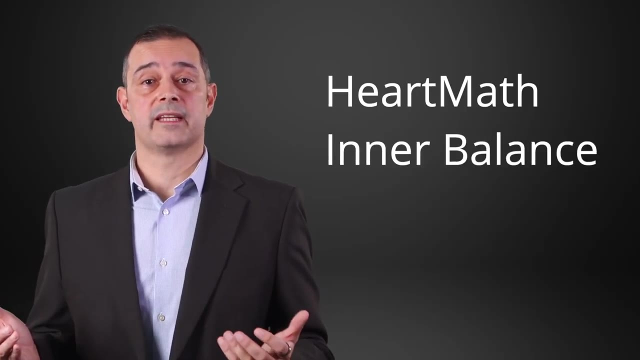 This measures your HRV using your phone camera and it provides insight into your stress levels. I use this with my clients suffering from burnout, chronic stress and anxiety as a way to get objective insight into their wellbeing. If you want to use HRV to improve your stress levels, then you want the HeartMath Inner Balance.